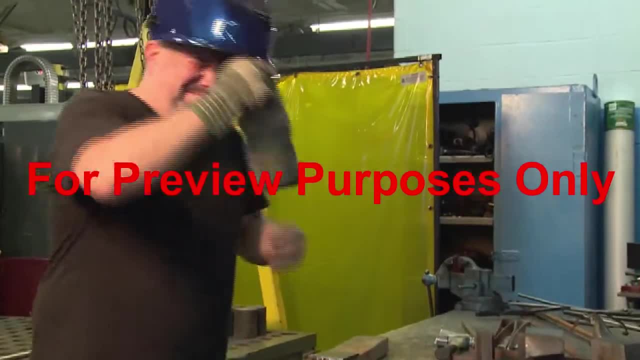 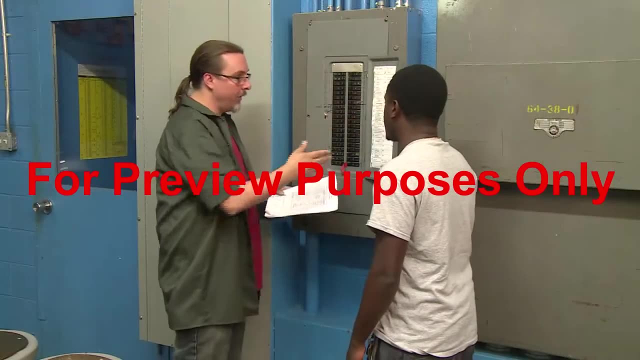 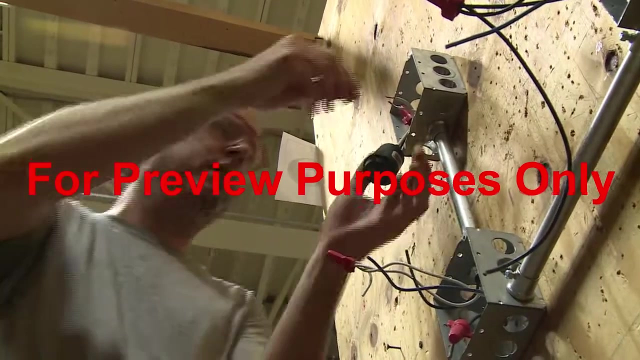 That can mean pain, injury, sometimes even death, So it's important to understand why these things happen. If we make each one a learning experience, we can prevent the same types of accidents from happening again. An accident can be caused by hazardous conditions or unsafe work practices, But even 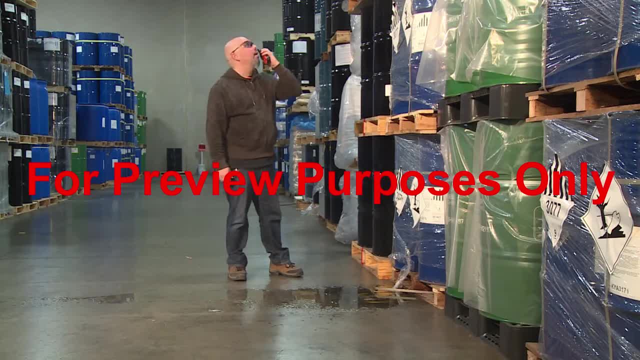 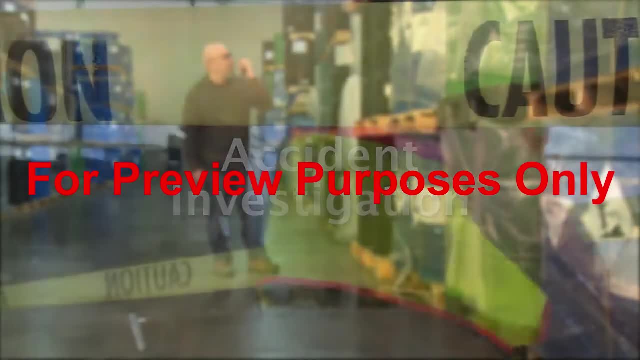 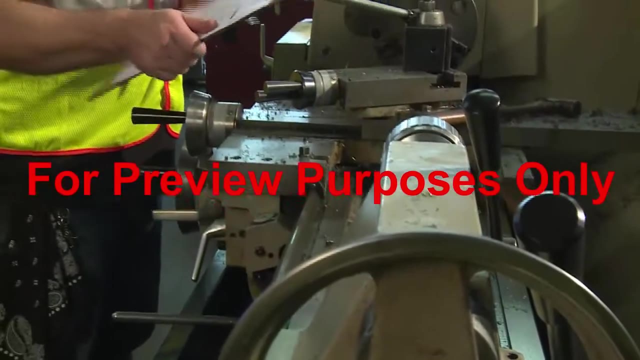 when the reason seems obvious, the real root cause can often be something else. That's where accident investigation comes in. It examines an incident systematically to determine its true causes. That information is then used to update policies, procedures or equipment to reduce the. 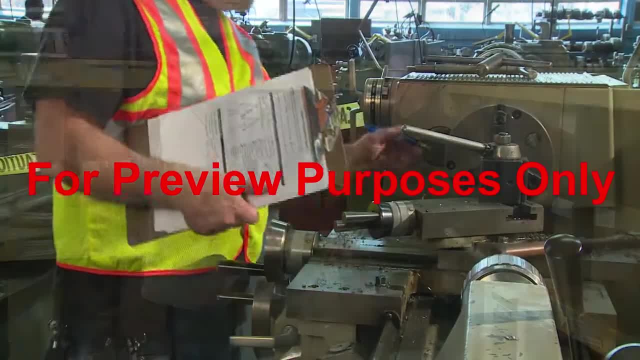 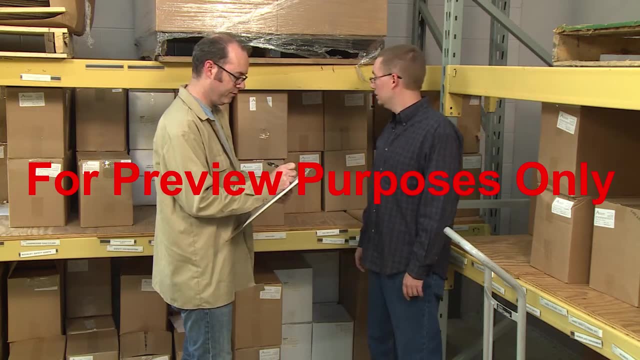 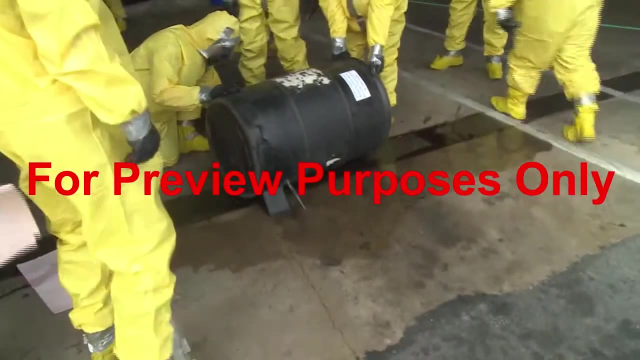 risk of that type of accident. The point of an accident investigation is not to assign blame or to get anyone in trouble. It's to prevent people from being injured in the same way in the future. But before we discuss the investigation, let's talk for a minute about how we 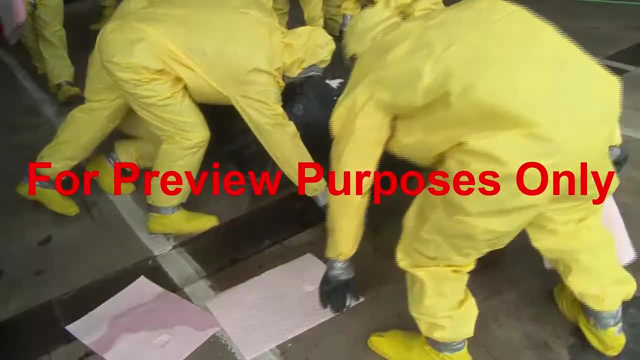 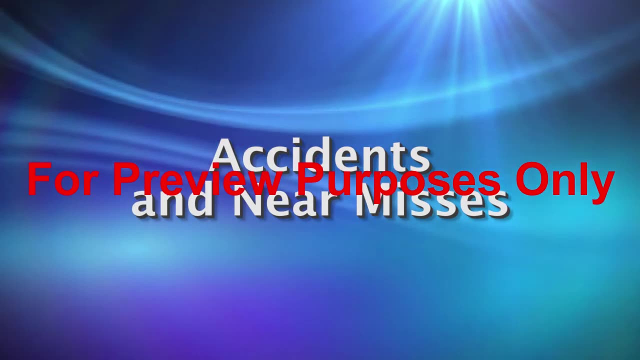 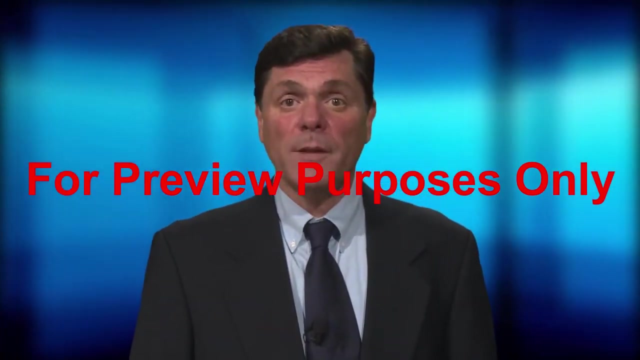 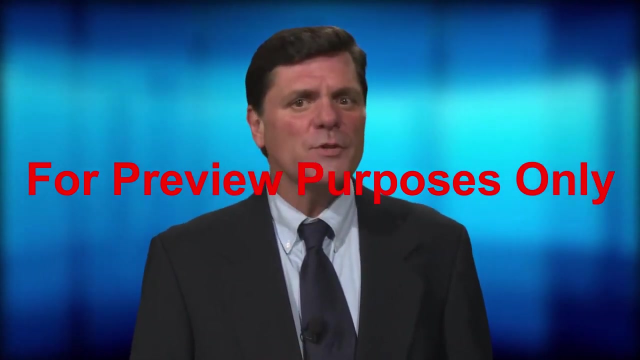 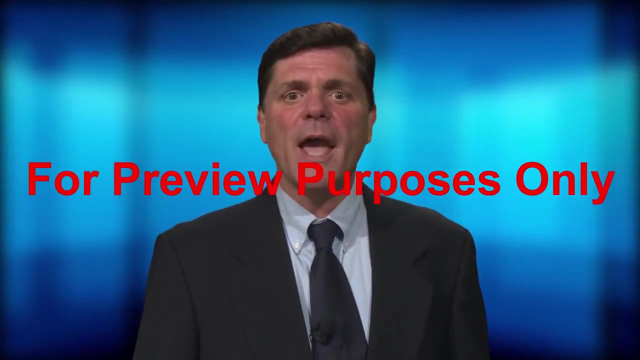 should deal with the incidents themselves. There are two types of workplace incidents: Accidents and near misses. A near miss is an incident which, under slightly different circumstances, could have resulted in an injury or damage to equipment or materials. In other words, an accident waiting to happen. 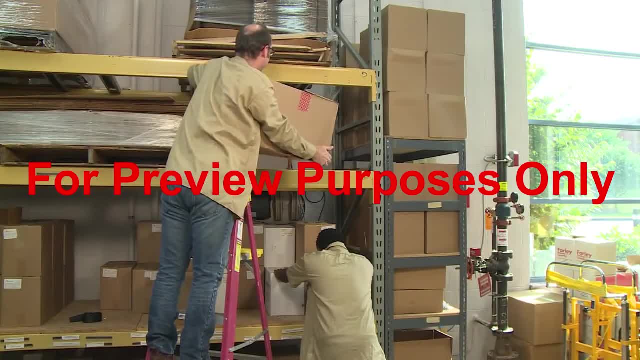 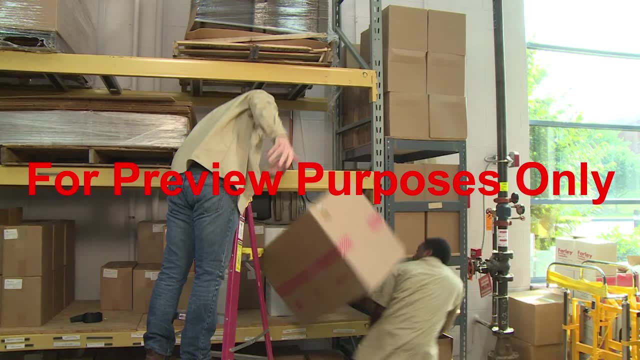 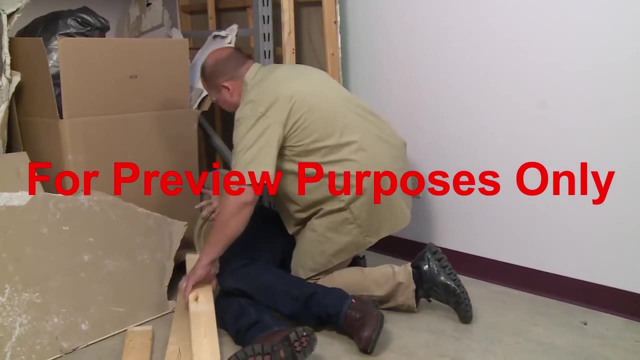 Near misses can warn us about a problem before something more serious happens, And it's much more likely to be an accident than an accident. And it's much better to learn from near misses than from accidents. Unfortunately, we won't always have a near miss to warn us about a potential problem. If an accident does occur, our first concern should be that the people who are injured are being cared for. 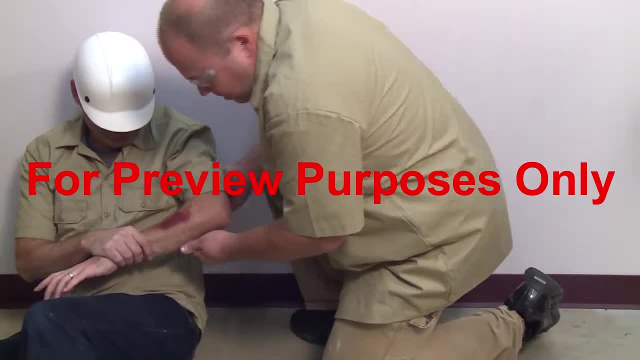 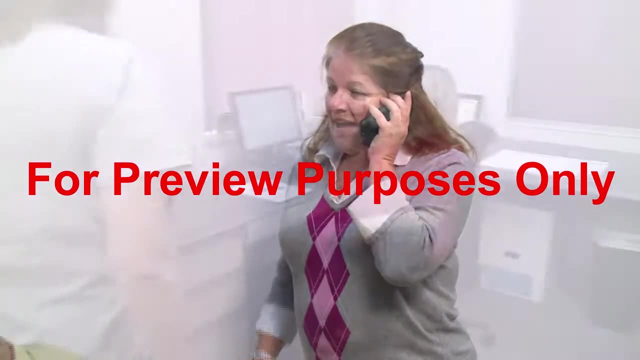 If someone needs first aid and you're qualified to give it, that should come first. Then medical personnel should be called immediately. Once any victims are taken care of, they should be called immediately. Once any victims are taken care of, they should be called immediately. 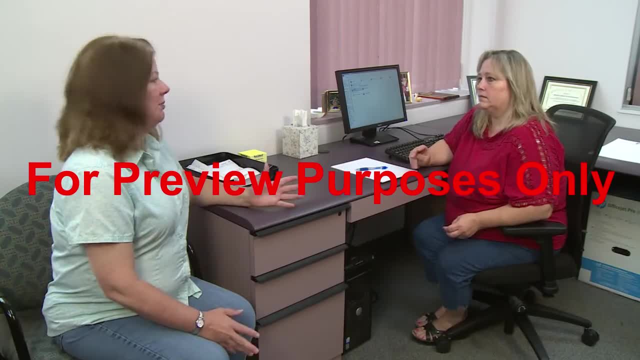 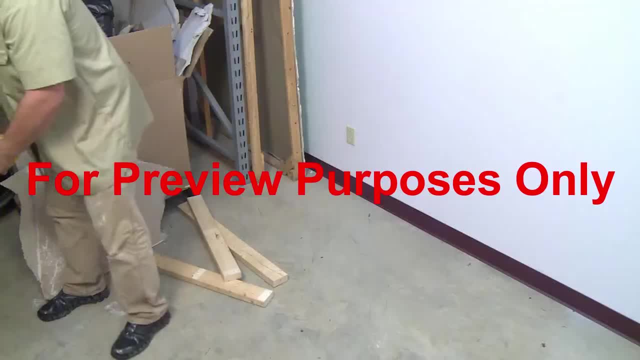 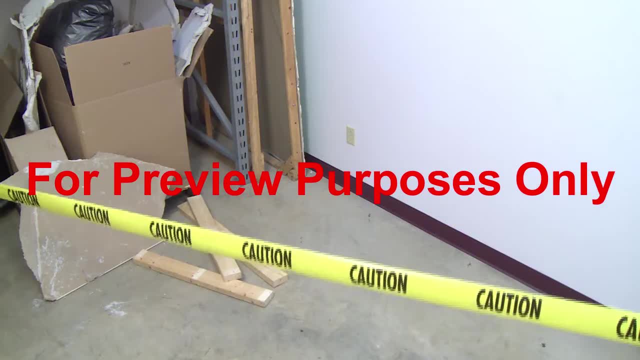 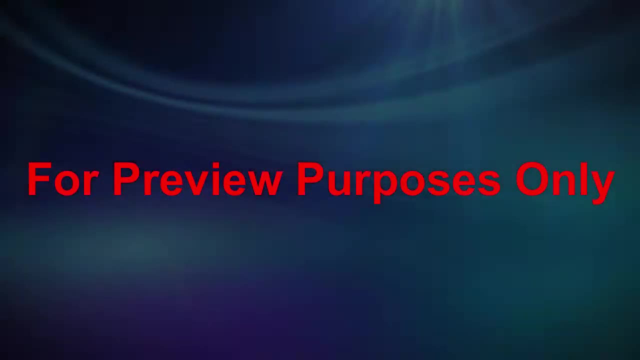 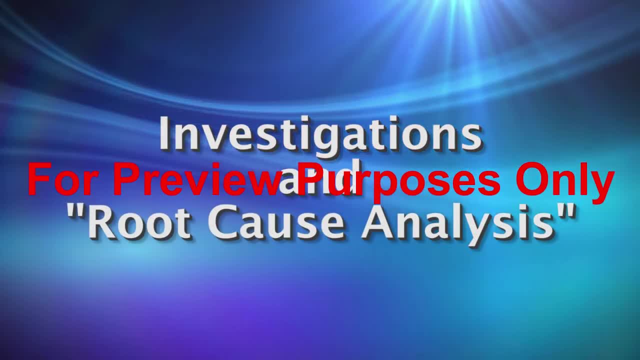 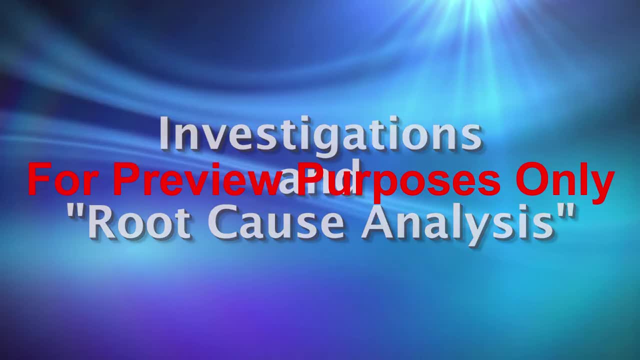 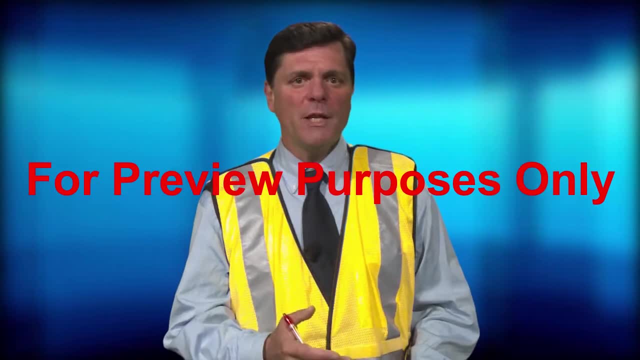 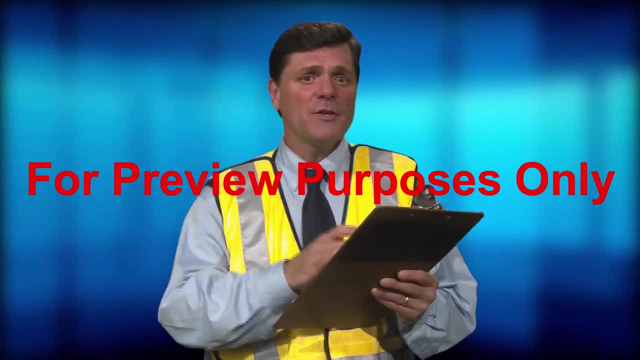 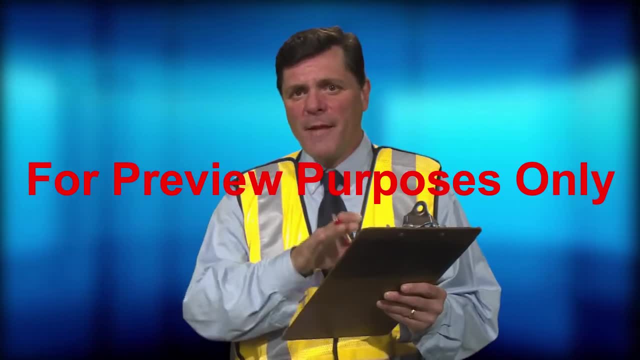 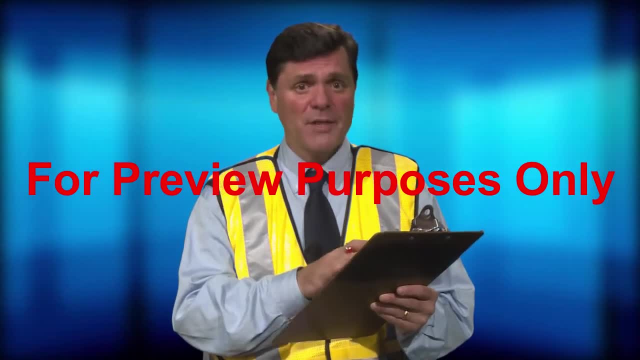 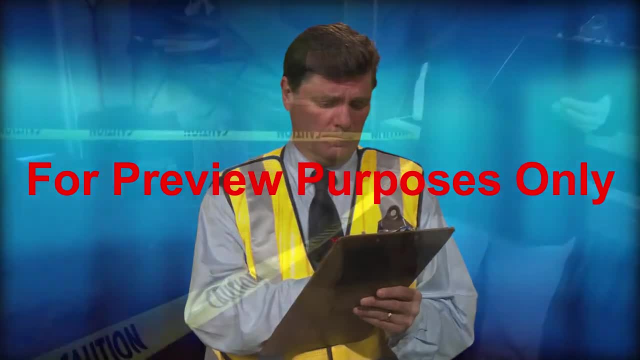 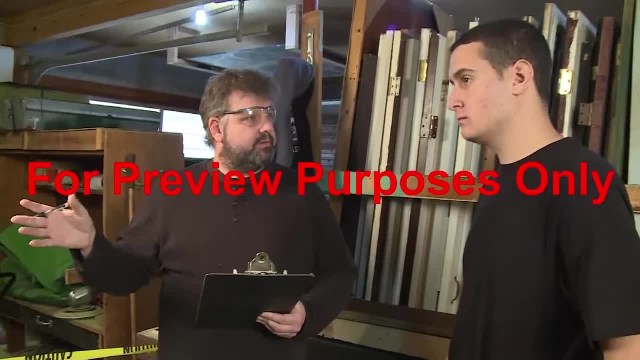 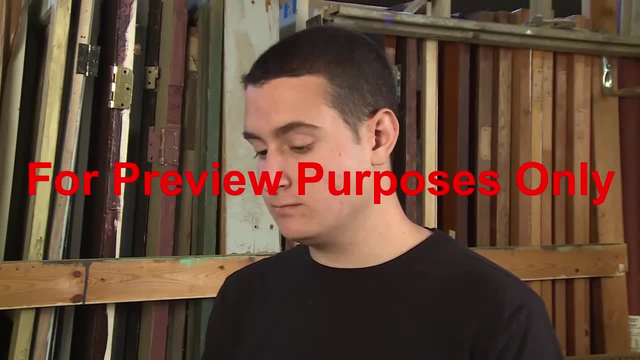 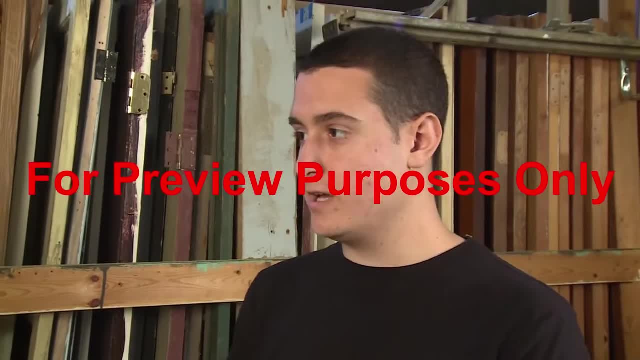 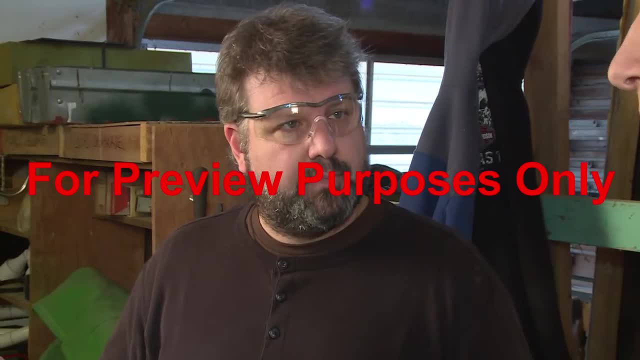 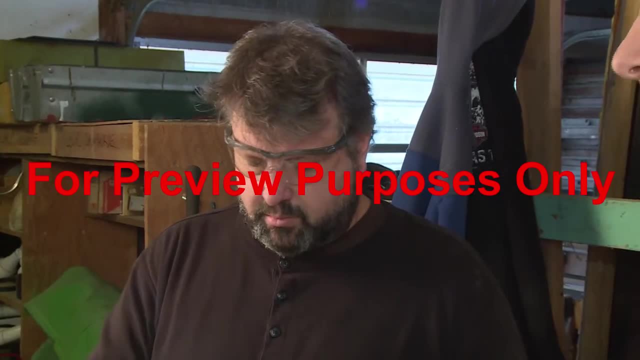 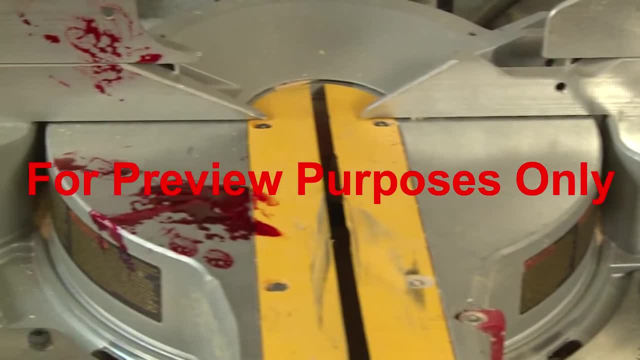 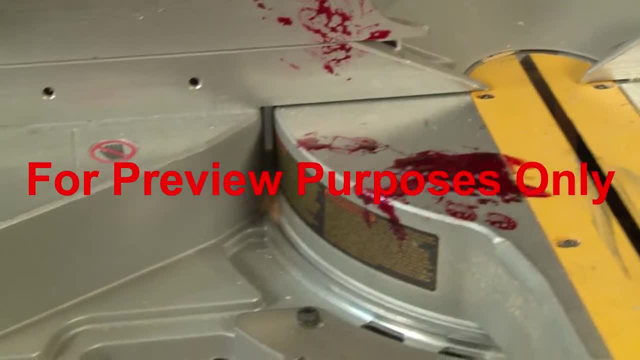 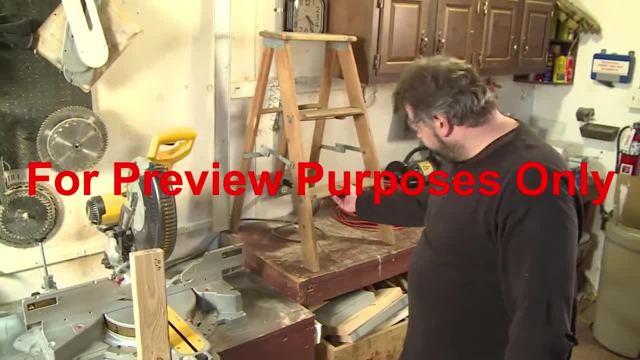 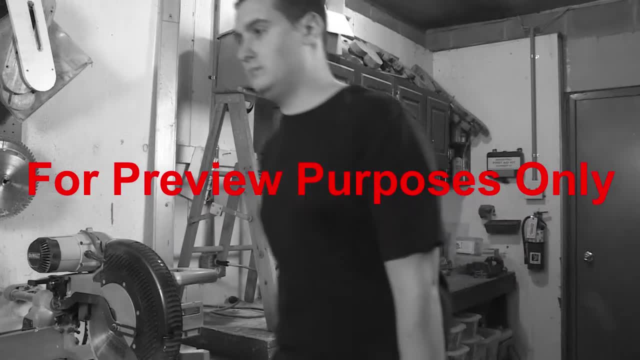 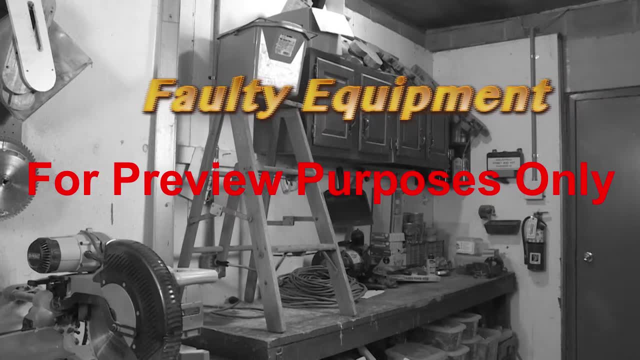 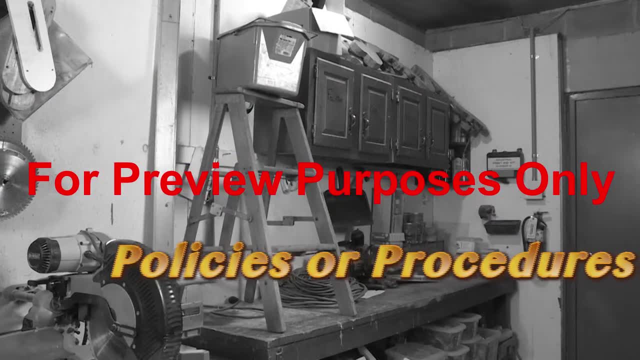 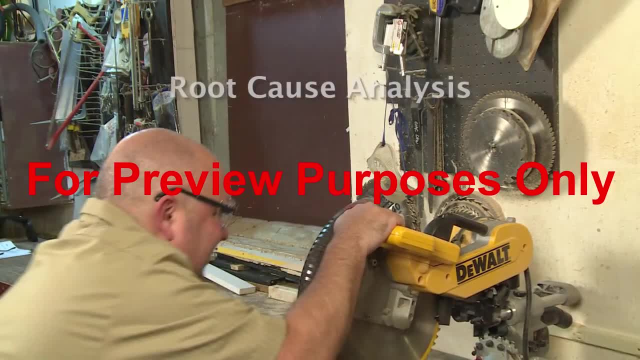 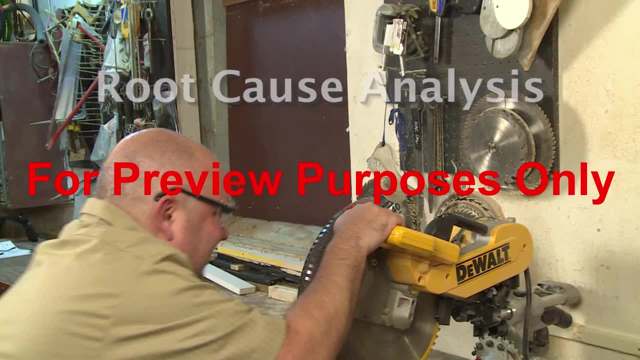 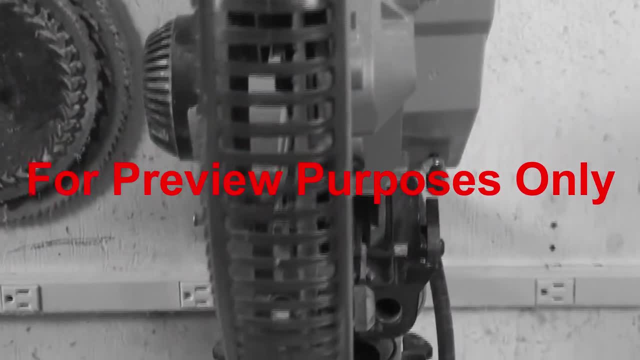 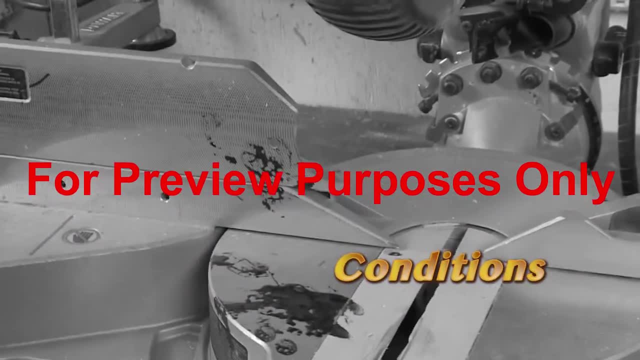 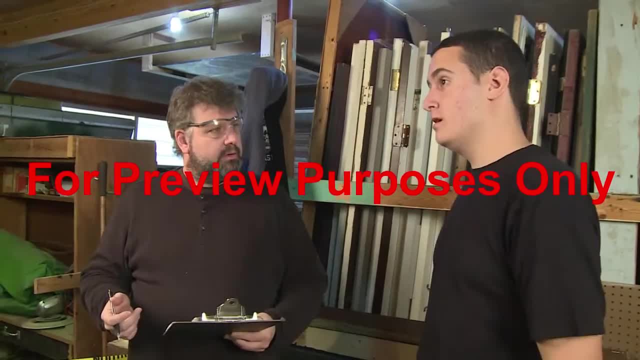 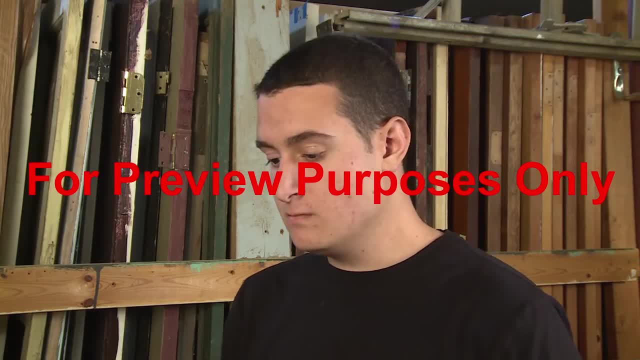 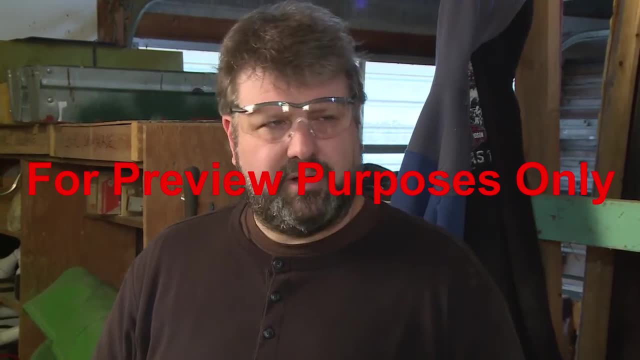 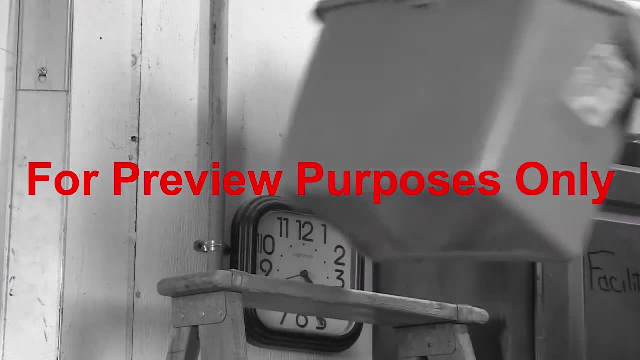 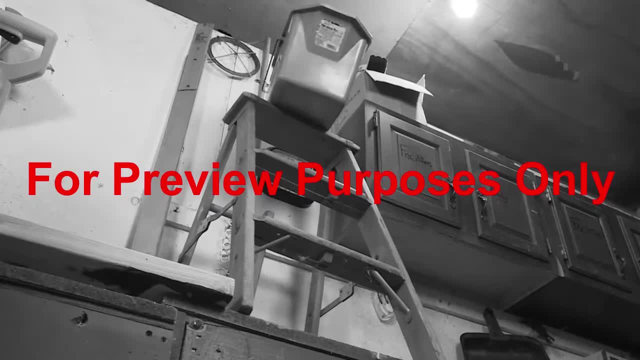 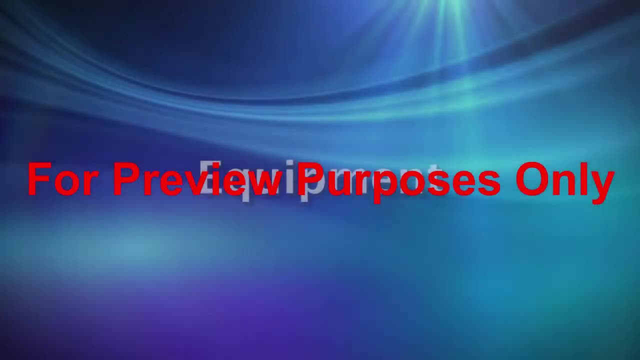 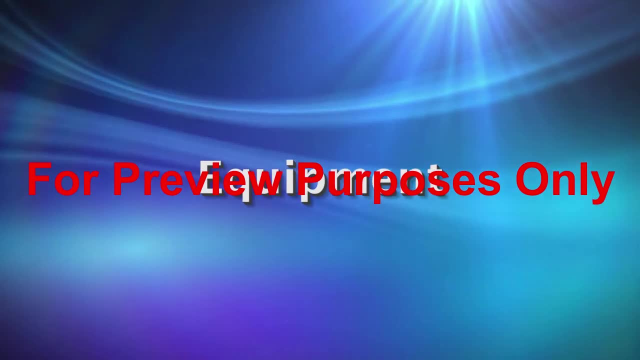 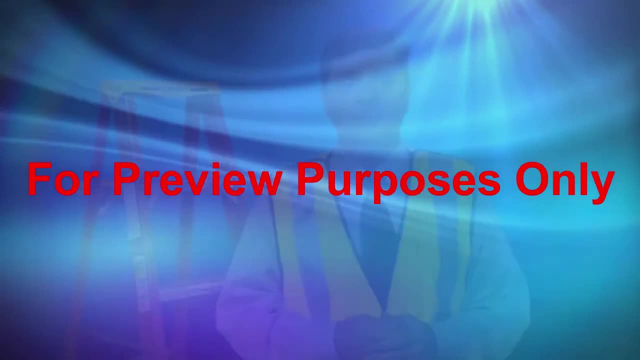 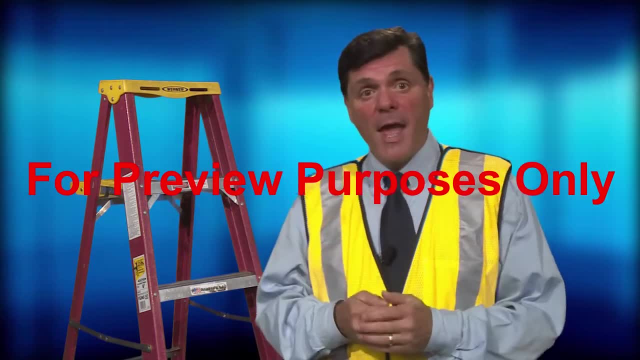 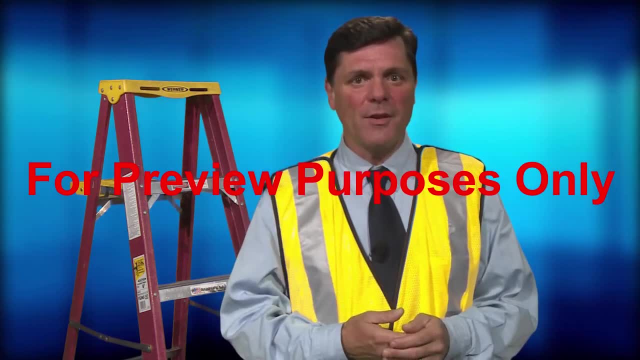 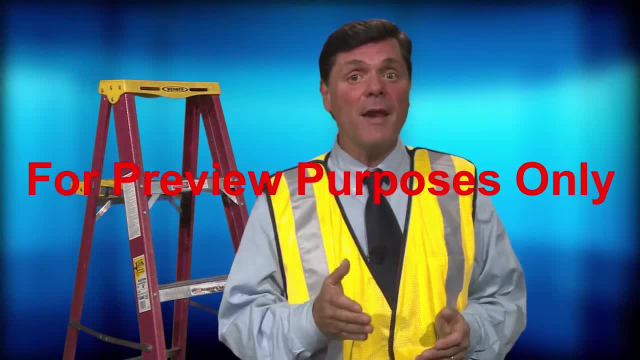 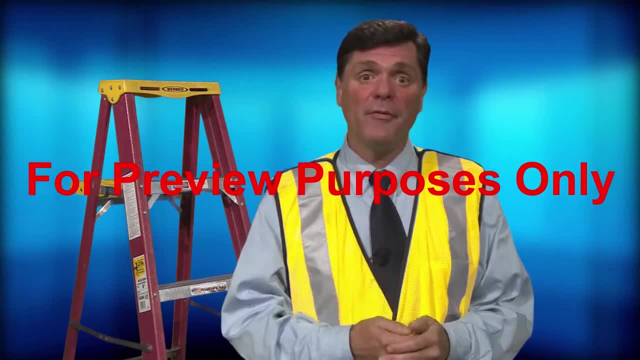 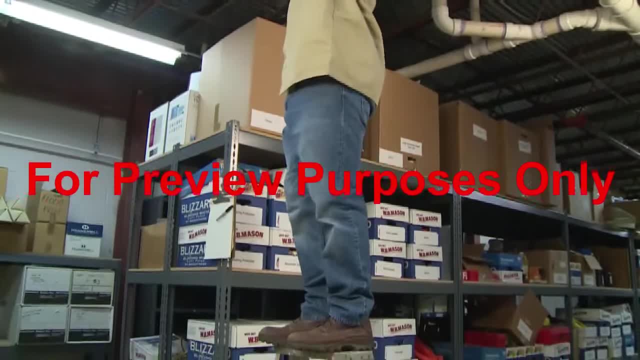 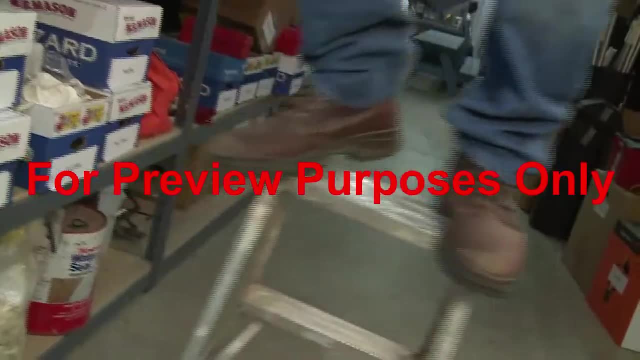 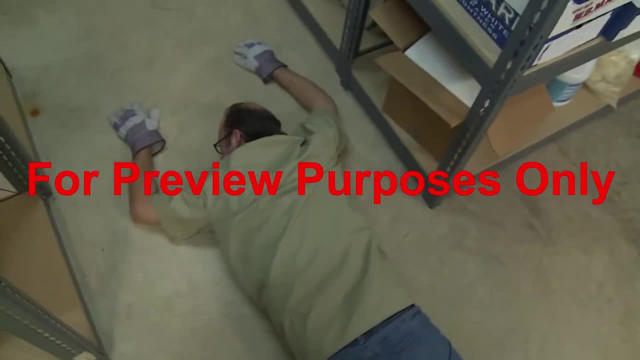 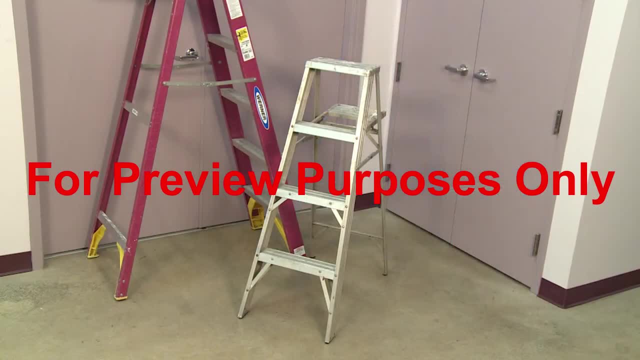 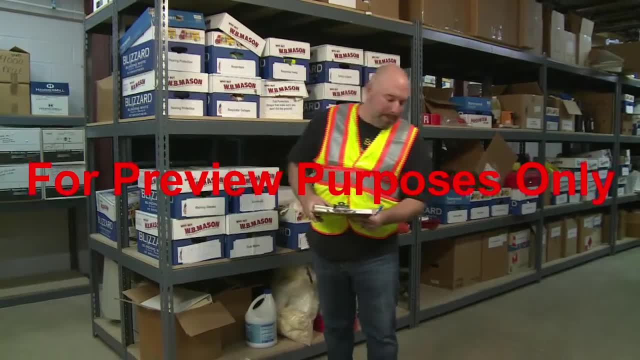 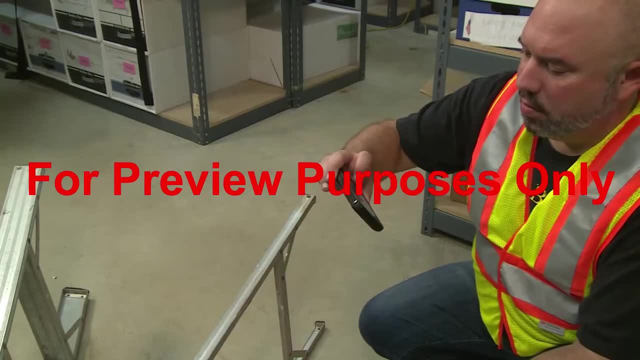 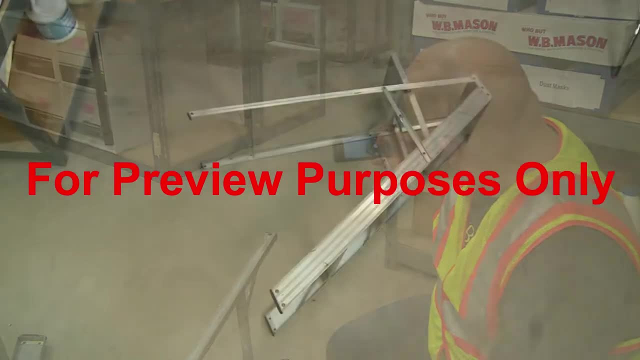 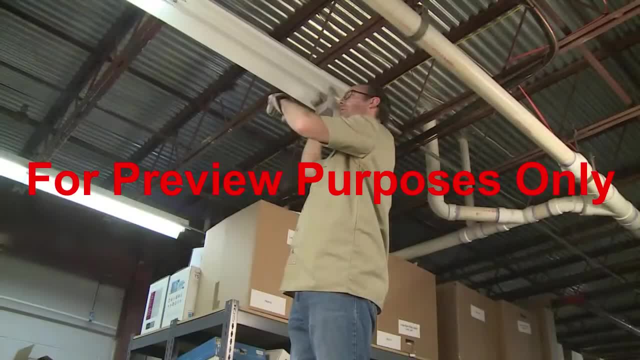 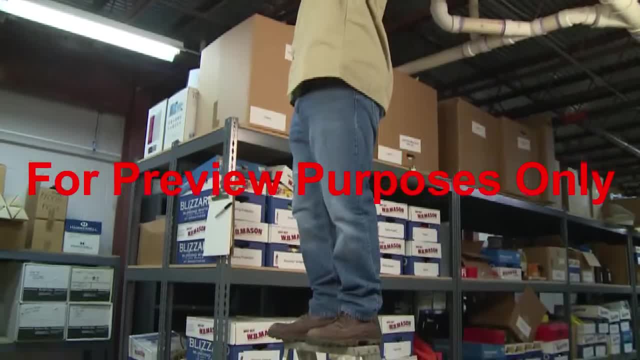 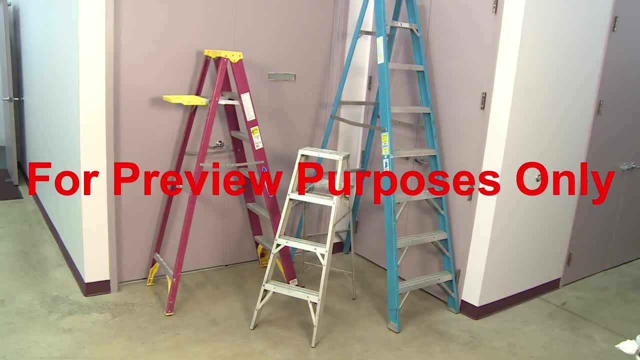 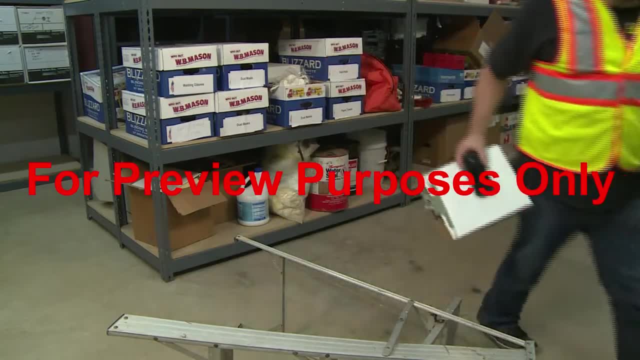 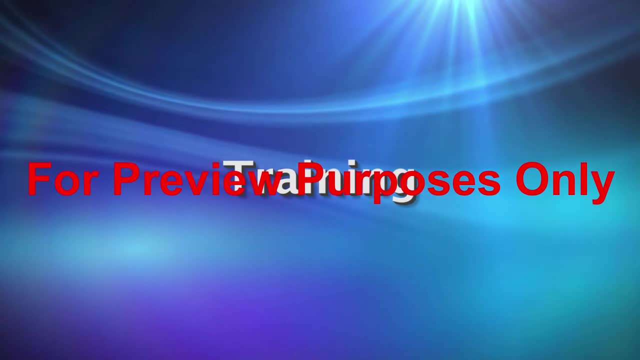 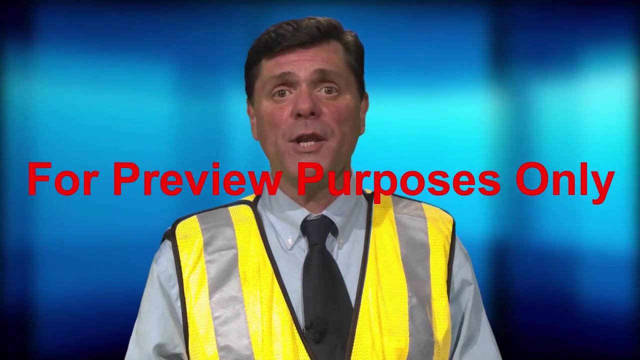 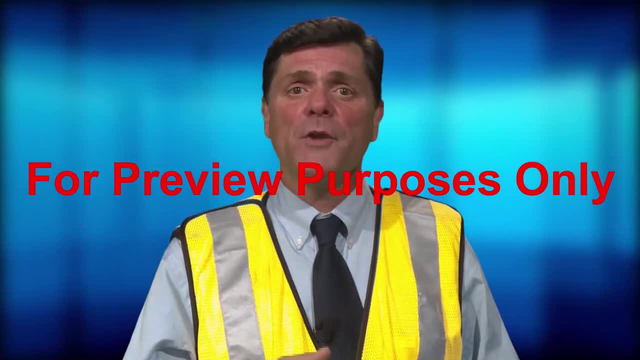 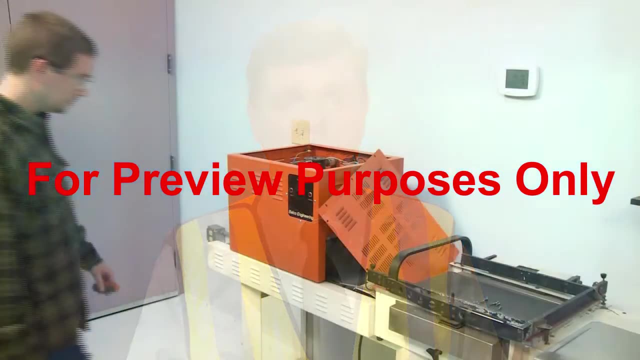 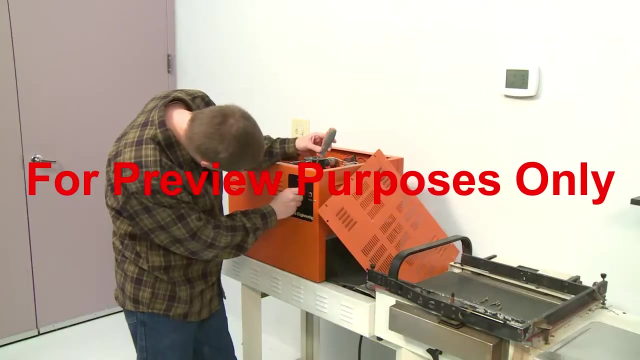 We might conclude that, since there was electricity involved, that the situation was inherently hazardous—that there wasn't much that could be done to make this situation safer. But it takes electricity to run the machine And there are procedures that allow electrically powered equipment to be worked on safely. 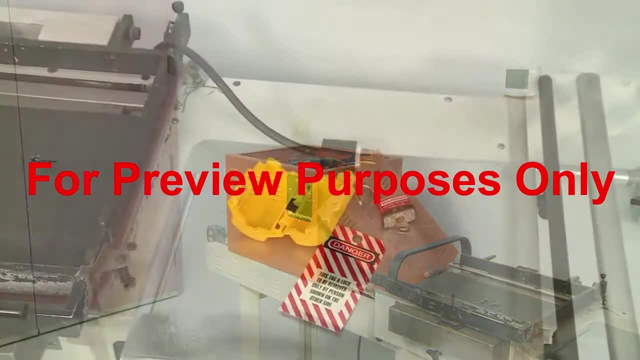 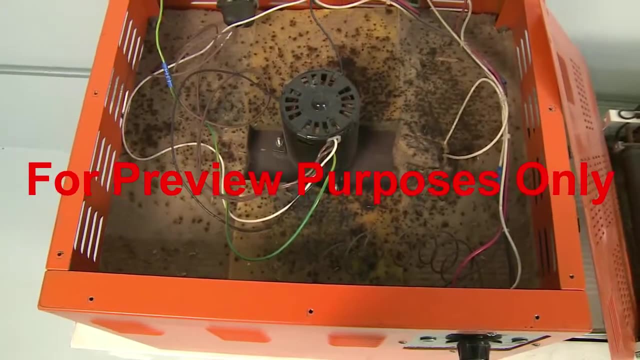 So there are probably other factors to consider. For instance, should the system have been locked out? If so, why wasn't it? We need to look at whether the worker who was repairing the machine had been given training on lockout-tagout procedures. 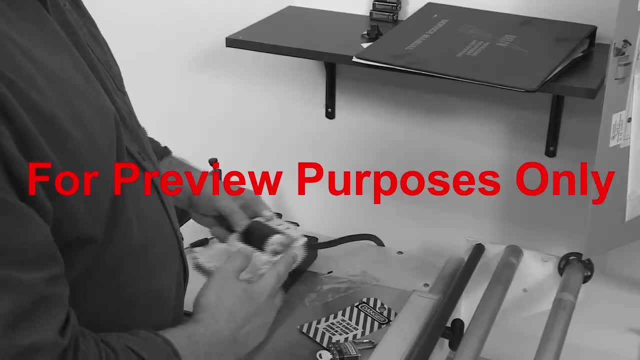 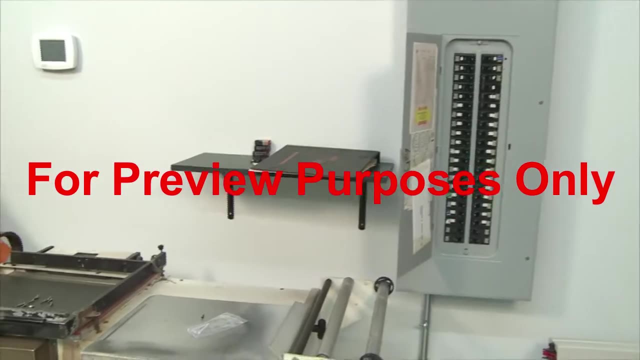 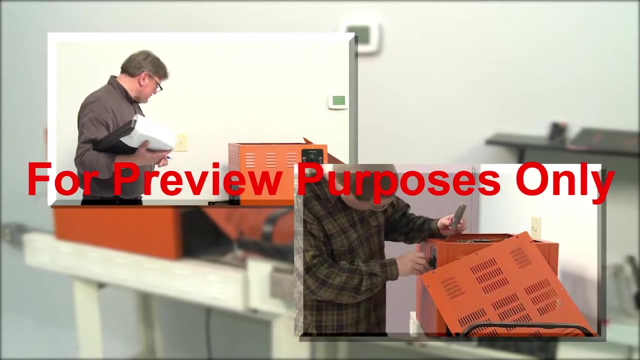 If he had received lockout-tagout training. we would also need to determine if the worker was following the procedures that he was taught. In this instance, the investigator determined that the root cause of the accident was a lack of training. The worker never attended the lockout-tagout class he was scheduled for and therefore never knew the danger he was putting himself into. 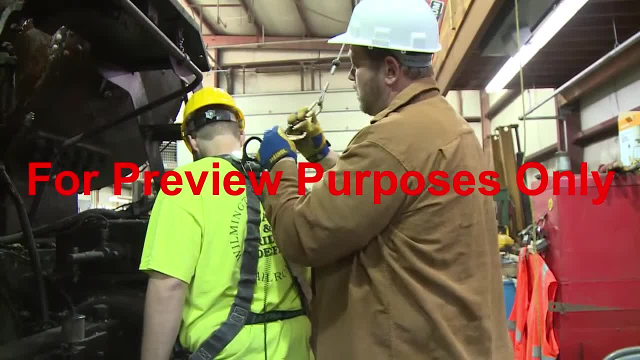 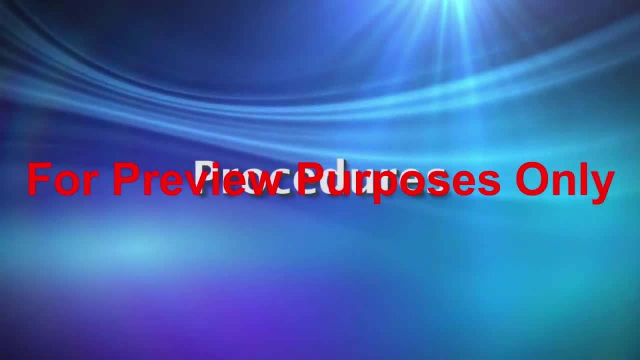 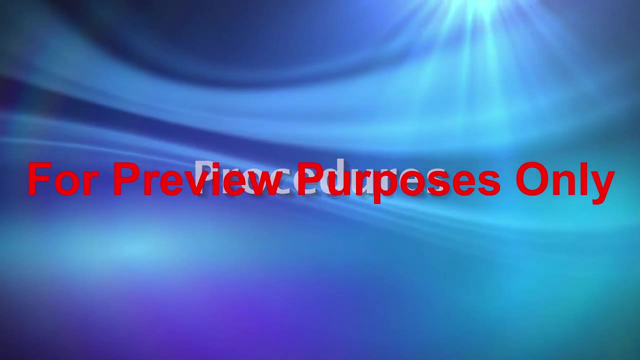 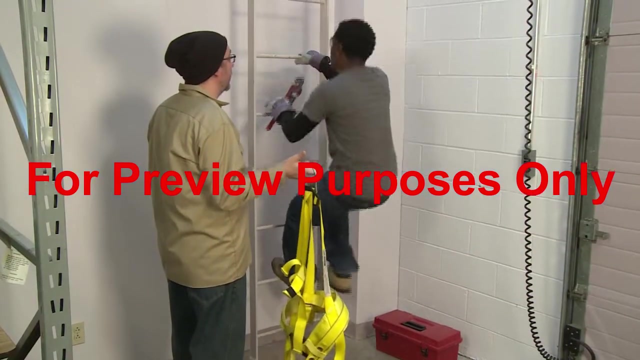 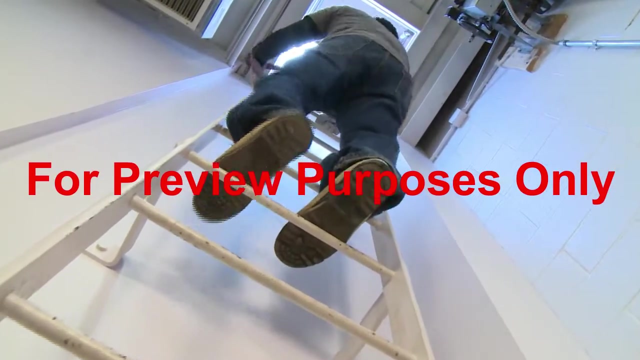 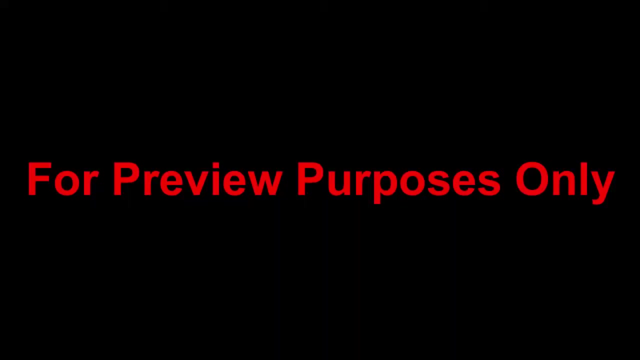 Now let's apply root cause analysis to a third situation, one that involves personal protective equipment. If a person falls, we usually figure they lost their grip or their footing, But when we take a closer look, In this case, we discover that the worker did not follow the instructions. 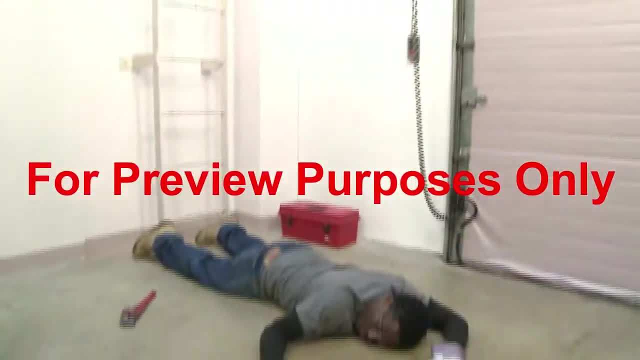 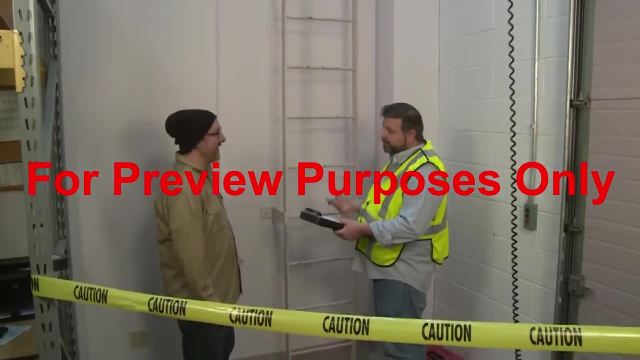 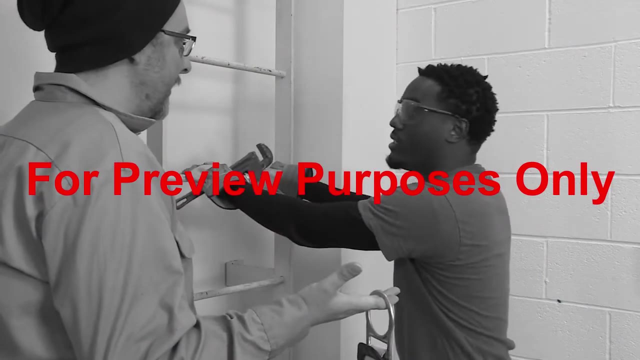 The worker did not follow procedure by wearing his fall protection gear. We would then need to find out why. There are a number of reasons why an employee might skip proper safety procedures- all of them bad- In an attempt to increase their output. a worker in a hurry can sometimes forget about safety. 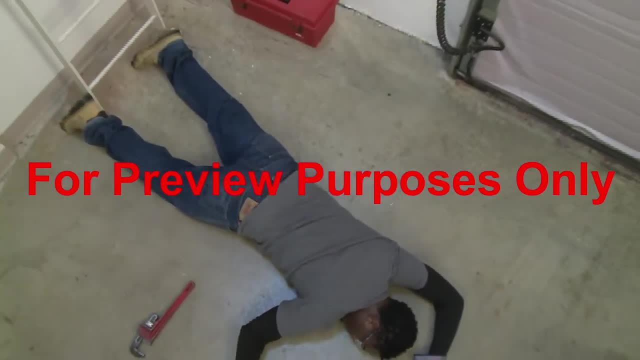 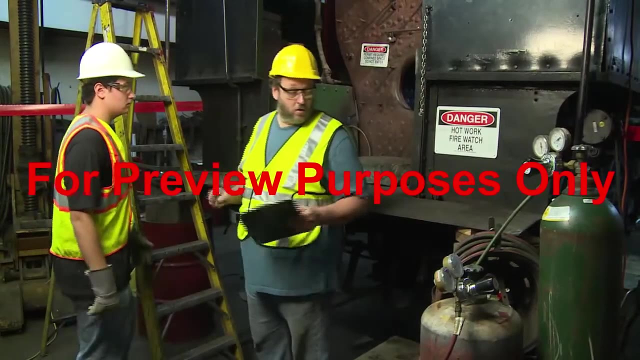 Ironically, if an accident occurs, as a result, production will often slow down or even stop altogether. There are times when an accident has nothing to do with safety. There are times when an accident has nothing to do with equipment, training or procedures. 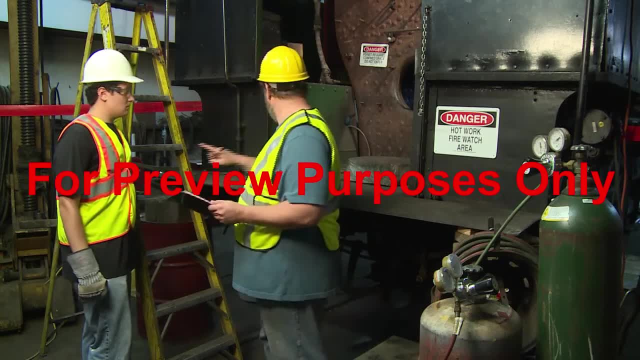 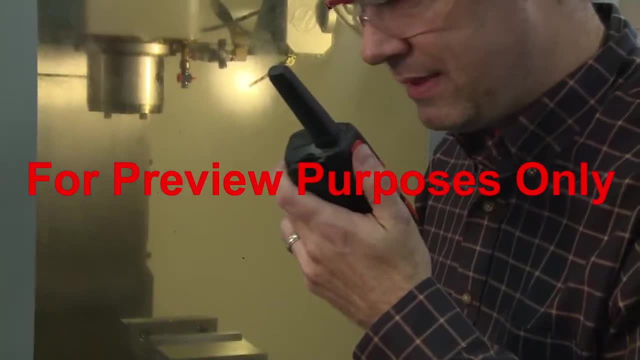 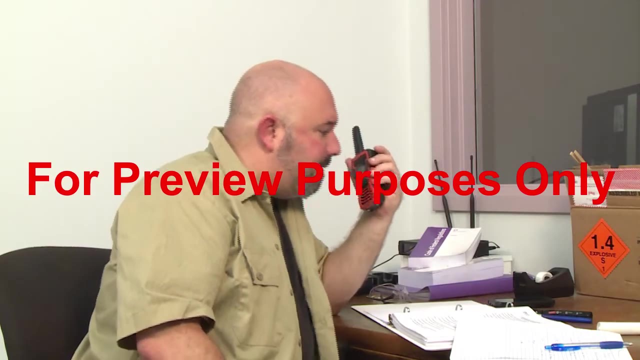 Often, investigators find that miscommunication is the root cause of an accident. Workers need to clearly hear and understand any instructions they receive about the job they're doing. If communications aren't clear or there is a question about what should really be done, instructions should be repeated so that everyone understands the proper procedure. 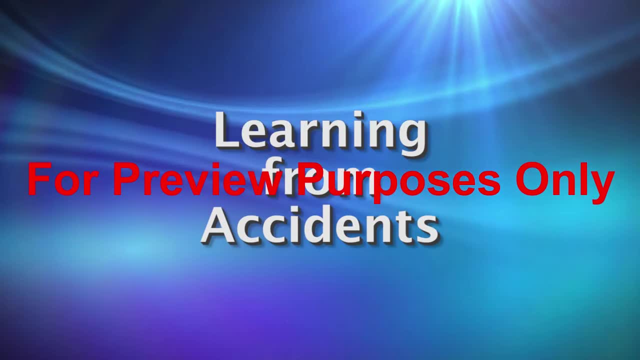 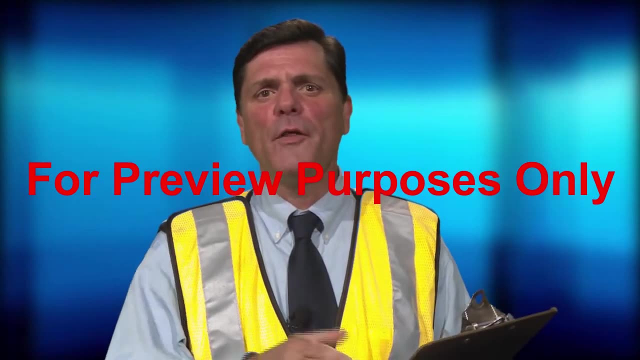 There are times when an accident has nothing to do with safety. There are times when an accident has nothing to do with safety. There are times when an accident has nothing to do with safety. So far, we've only looked at the first goal of an accident investigation: determining the cause. 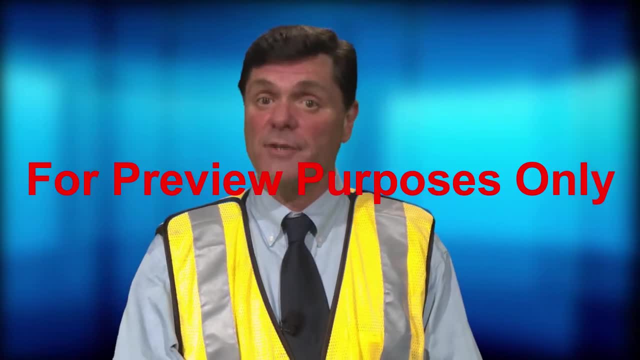 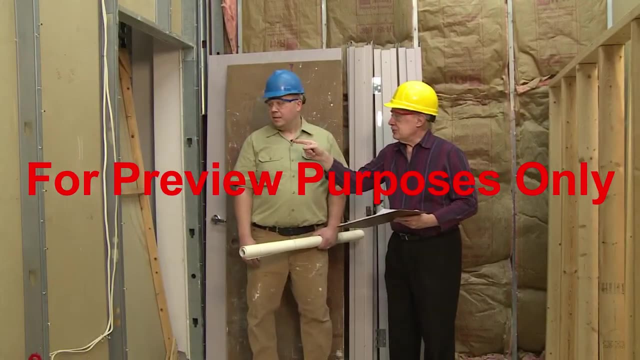 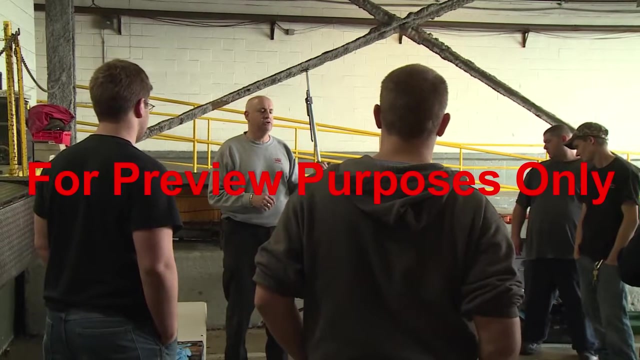 Now let's look at the other goal: making sure that the same type of accident doesn't happen again. Remember, when it comes to learning from accidents, there are four basic areas to look at: Policies, Training, Equipment and Communication. Proper training is always a key element in preventing accidents. 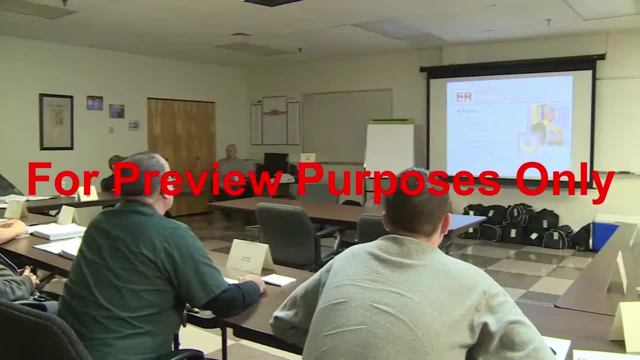 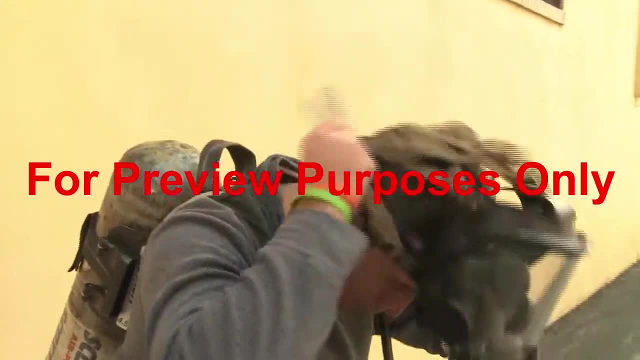 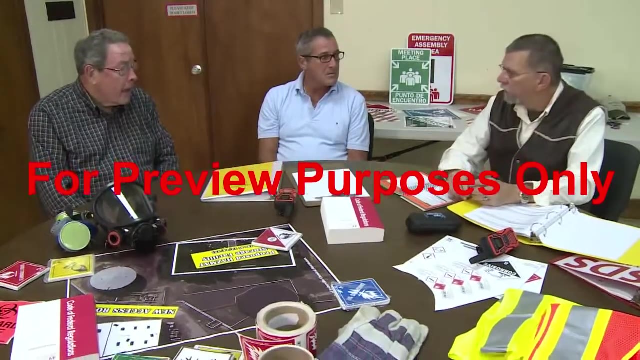 If problems have existed with certain types of activities or situations in the past, everyone should be made aware of the potential hazards that are associated with those situations and be trained to handle them. If a situation is hazardous enough, your facility may have to put new policies into place. 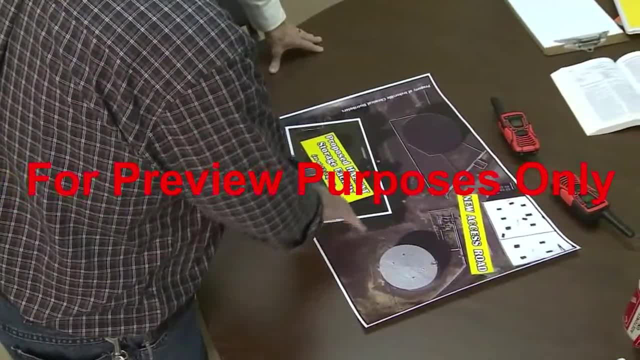 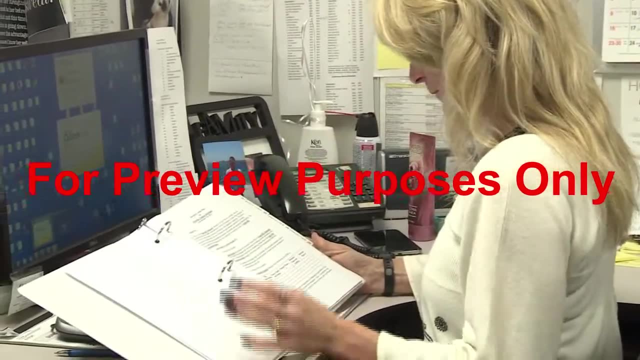 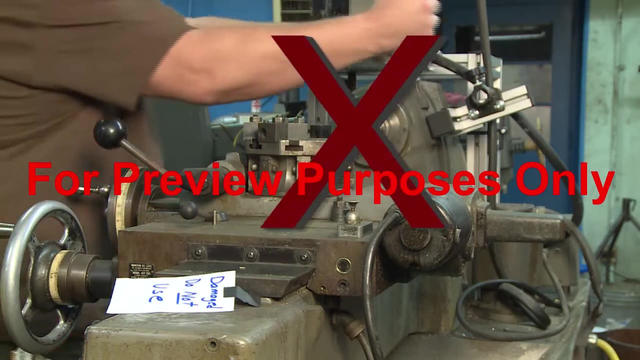 or existing policies. New policies may have to be updated. This can often take the form of workplace rules or standard operating procedures that everyone must follow. Many accidents are caused by faulty or misused equipment. In these cases, the equipment may need to be repaired.